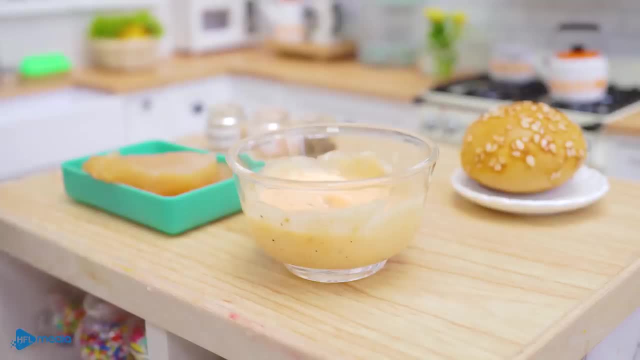 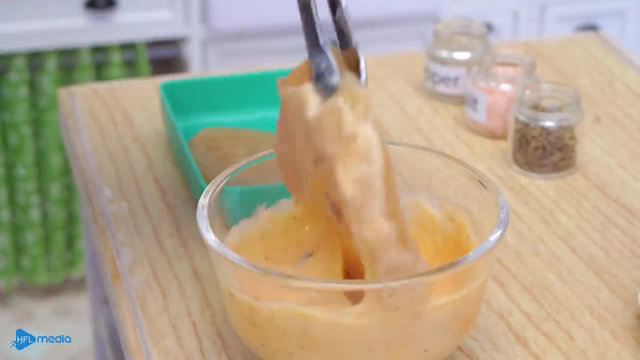 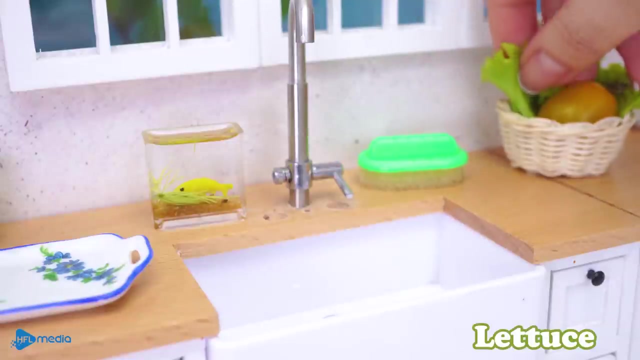 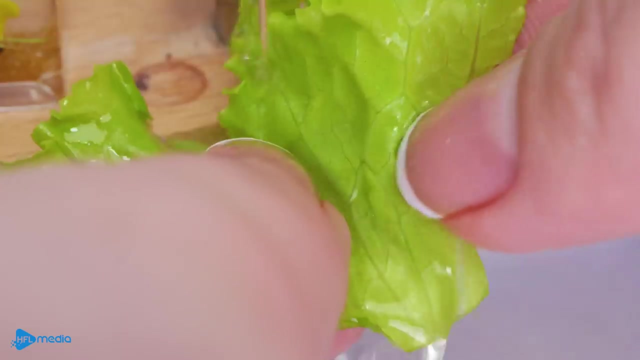 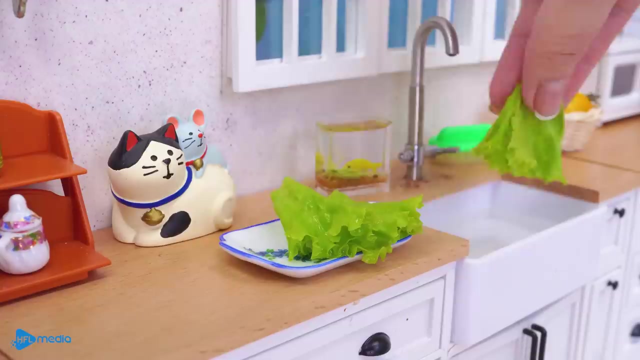 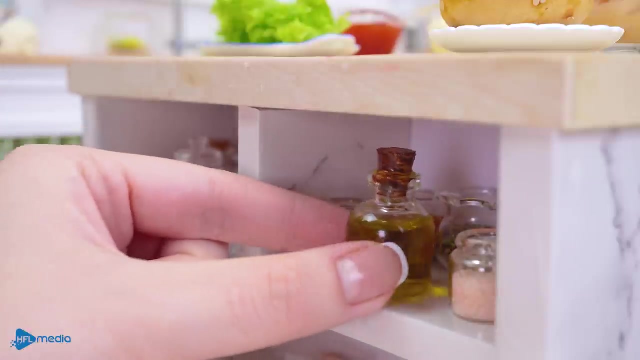 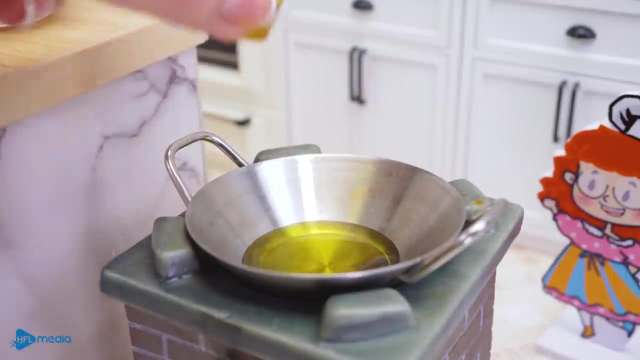 Mix well. Thank you for watching. Add 1 tablespoon of soy sauce, 1 tablespoon of sugar, 1 tablespoon of cooking wine and 1 tablespoon of cooking wine to the pan and stir-fry over medium-low heat. Add 1 tablespoon of cooking wine and stir-fry over medium-low heat. 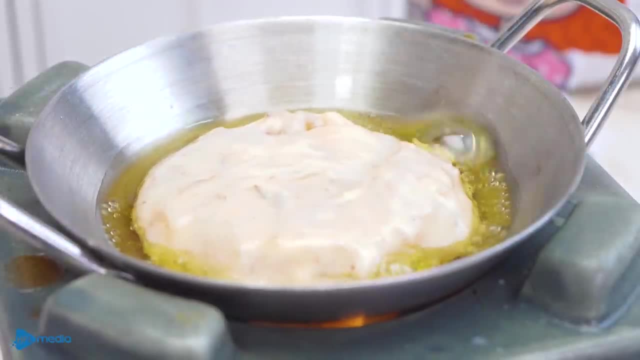 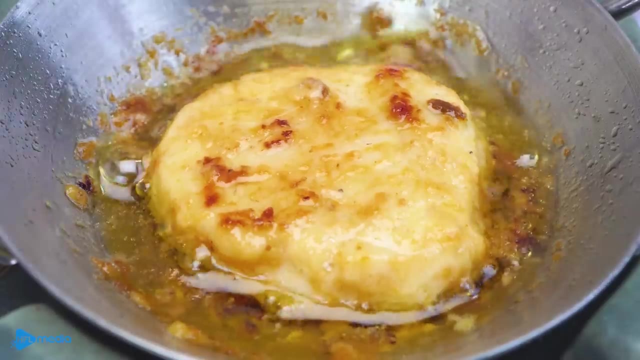 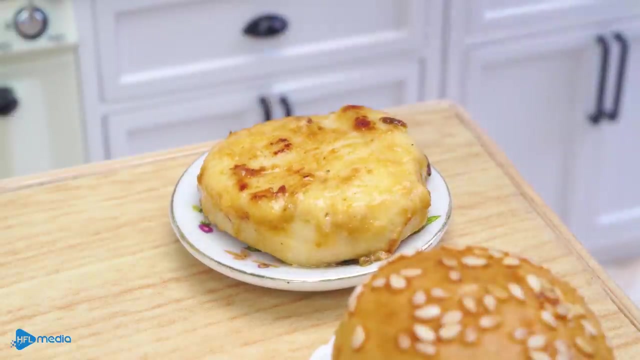 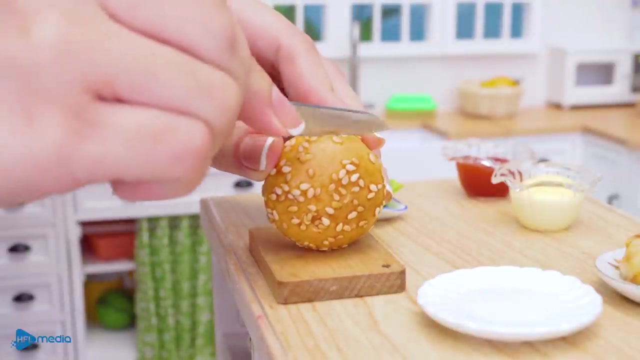 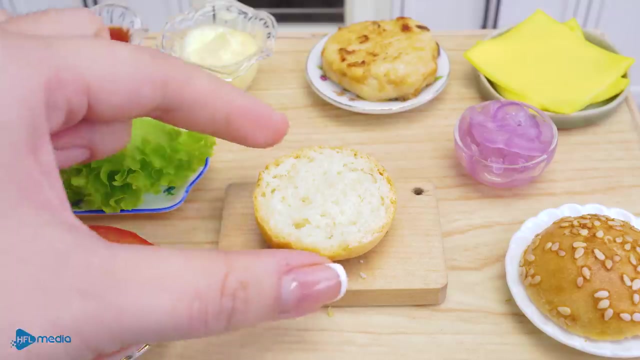 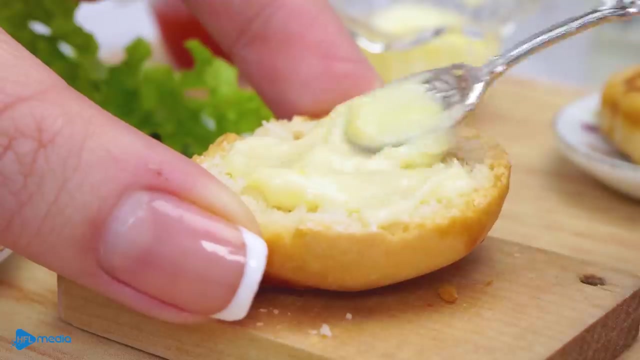 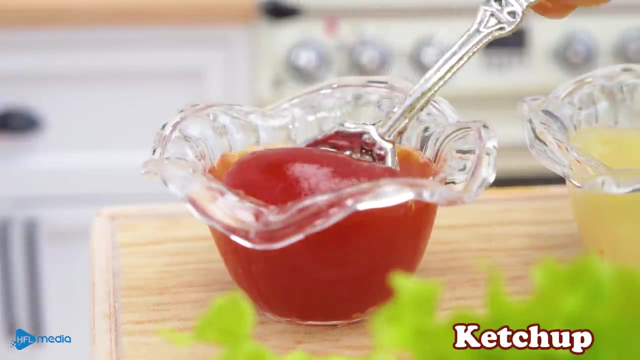 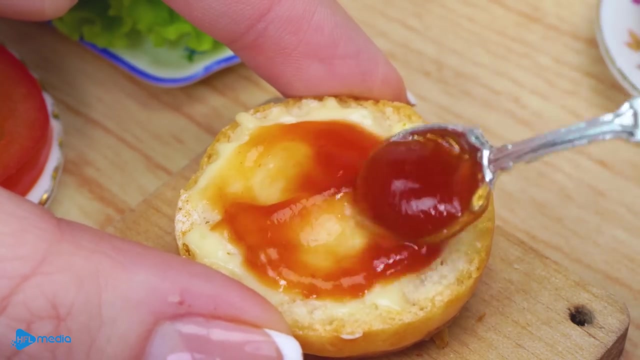 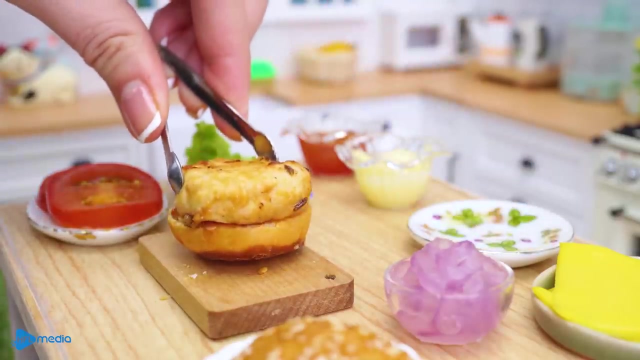 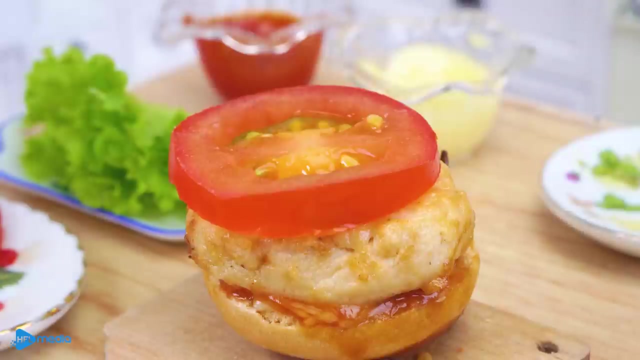 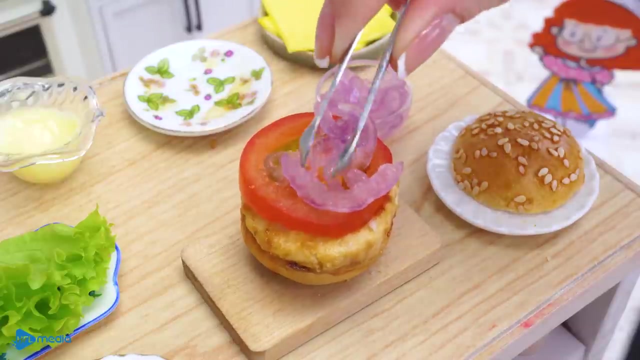 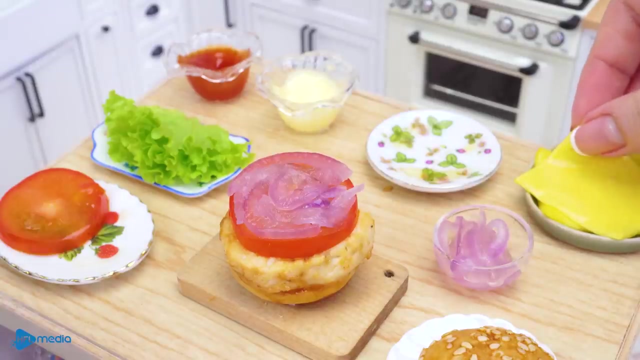 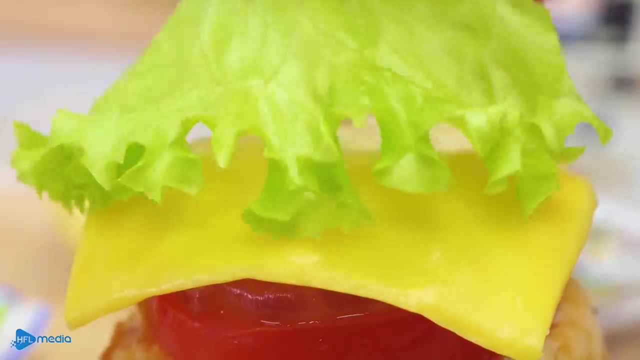 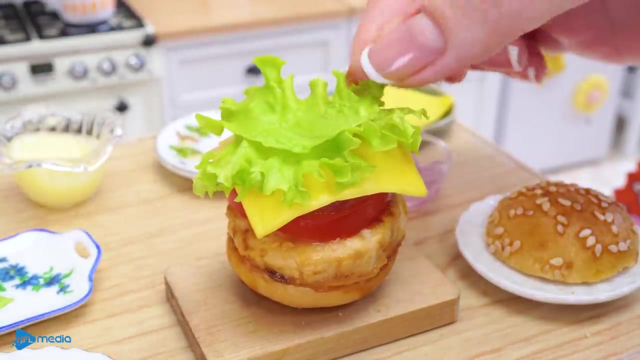 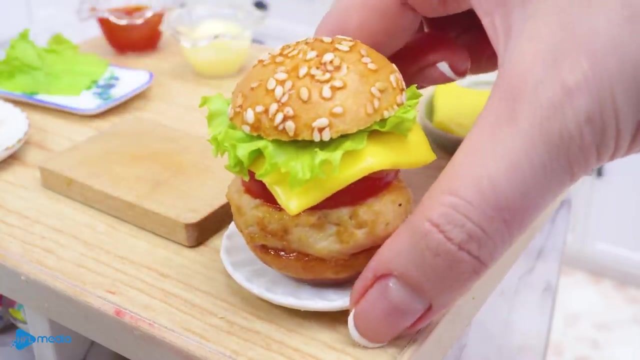 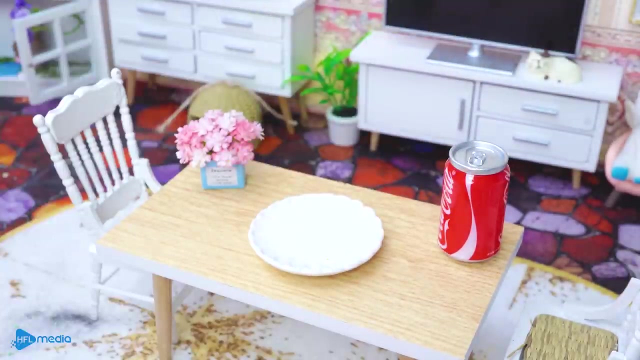 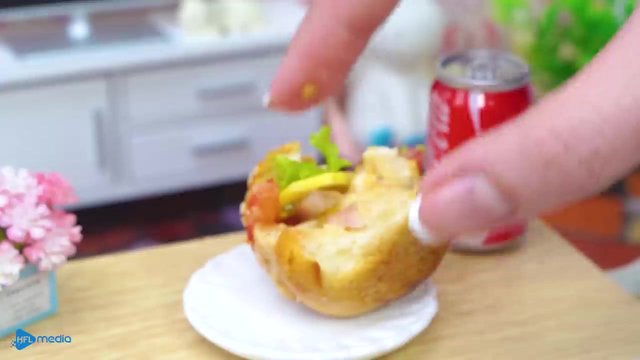 Add 1 tablespoon of cooking wine and stir-fry over medium-low heat. Add 1 tablespoon of sugar and mix well. Add 1 tablespoon of cooking wine and stir-fry over medium-low heat. Thank you, Thank you, Thank you. 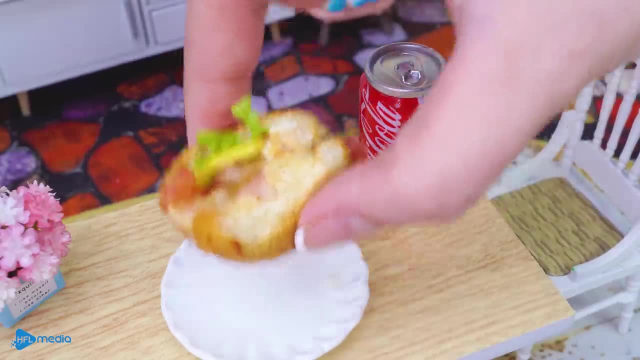 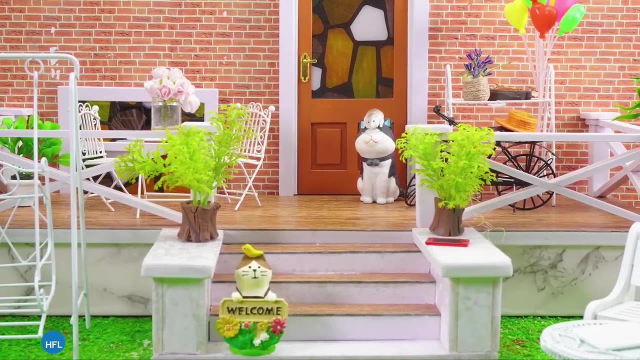 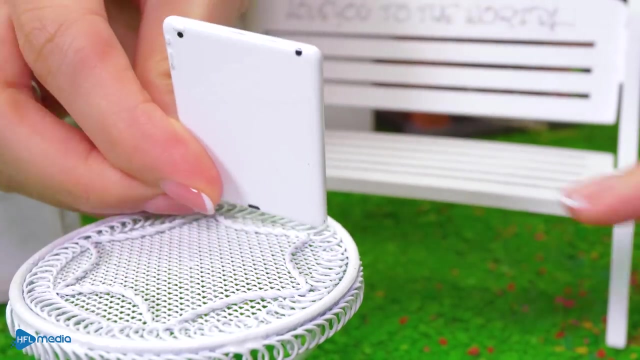 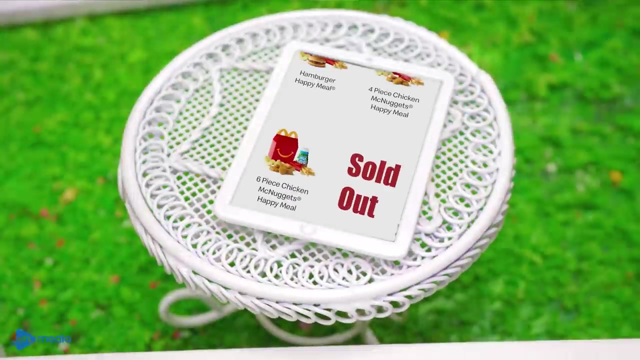 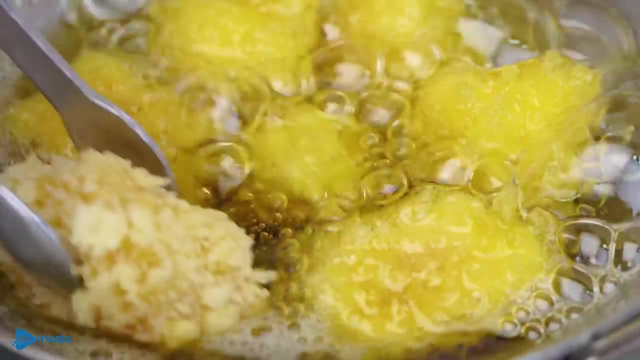 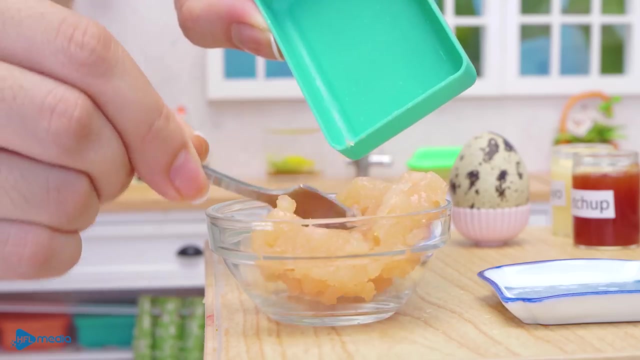 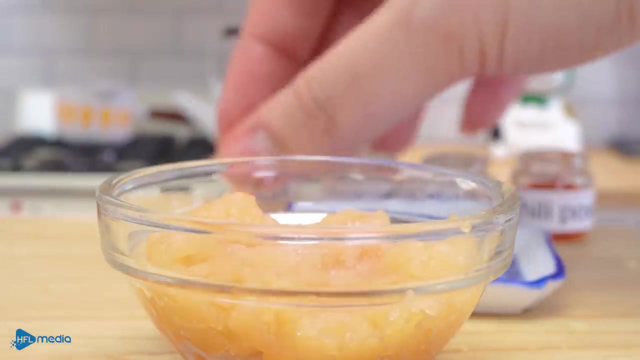 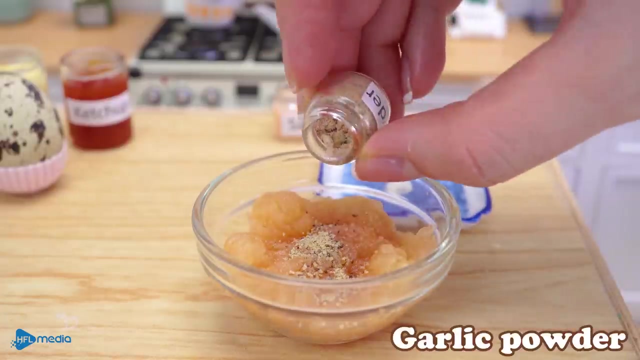 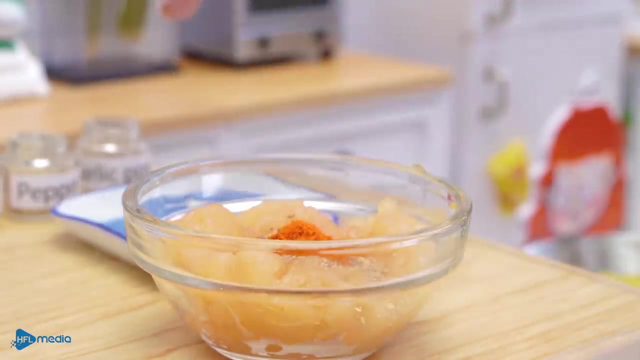 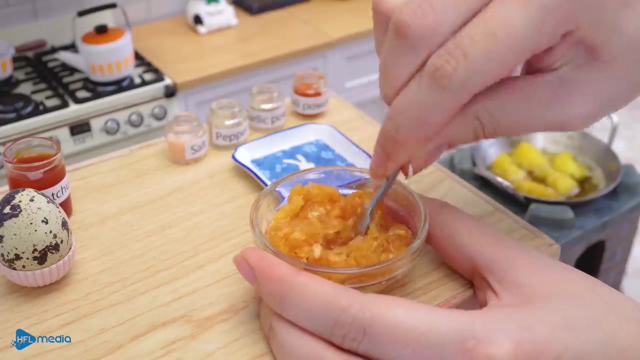 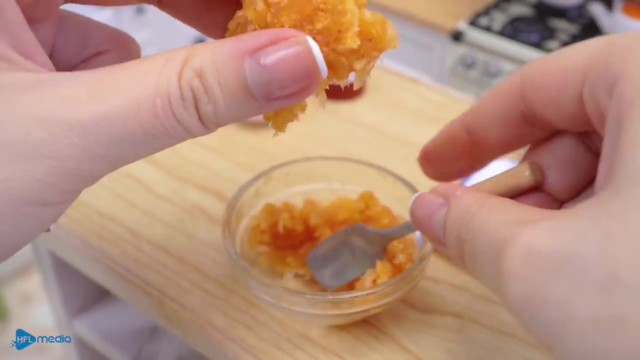 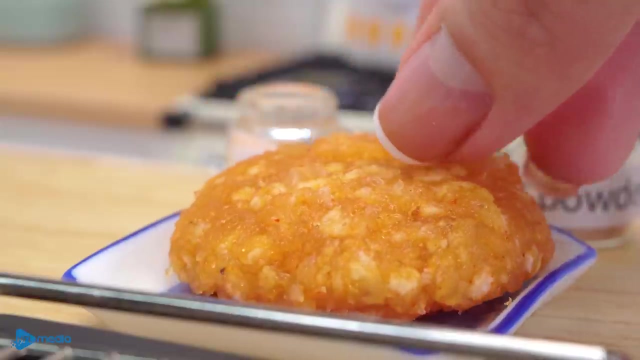 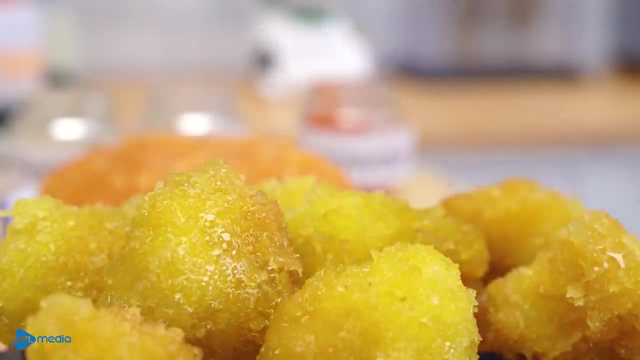 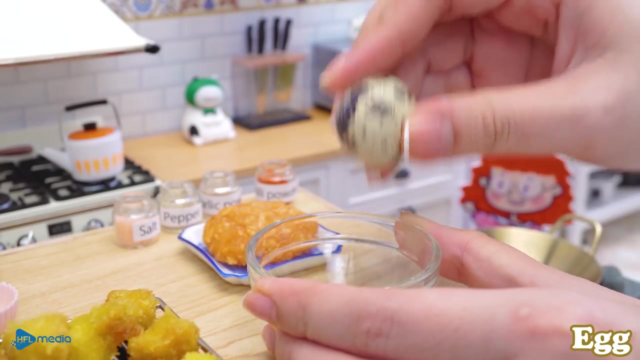 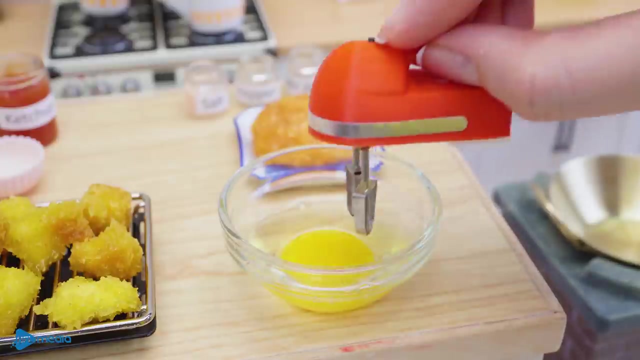 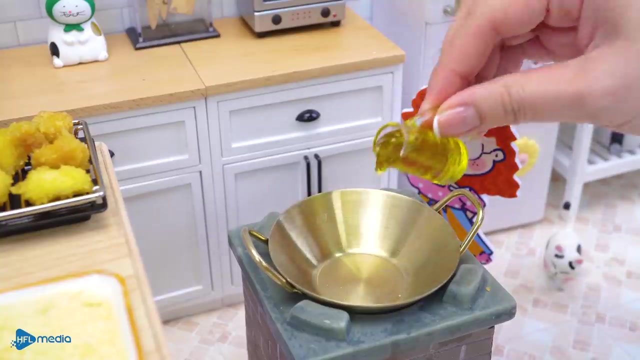 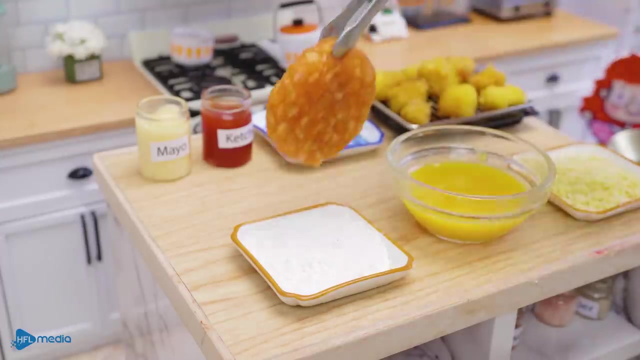 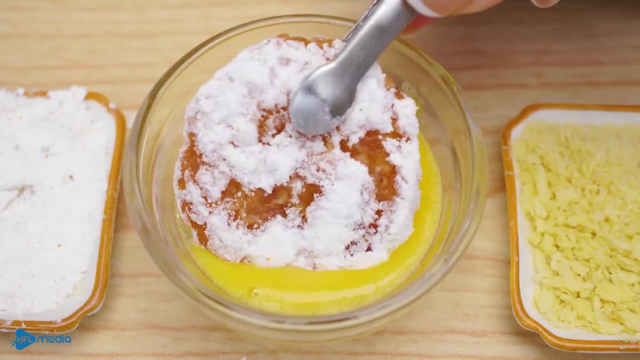 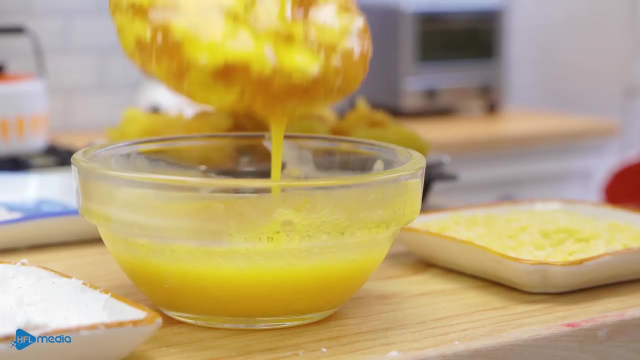 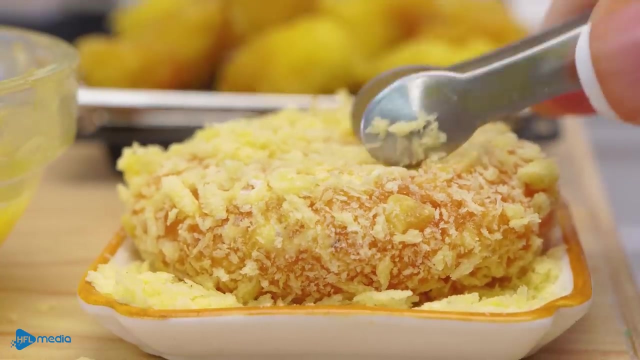 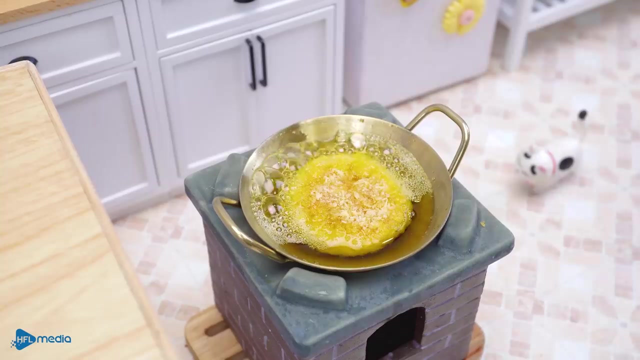 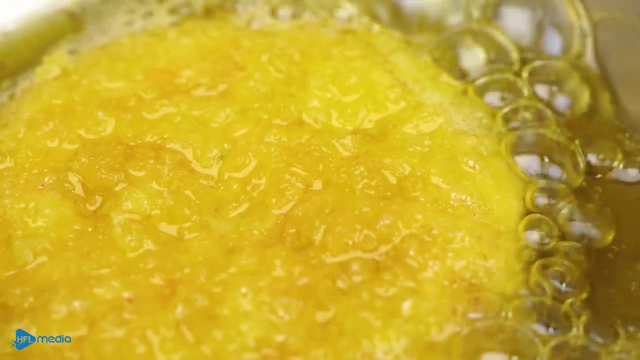 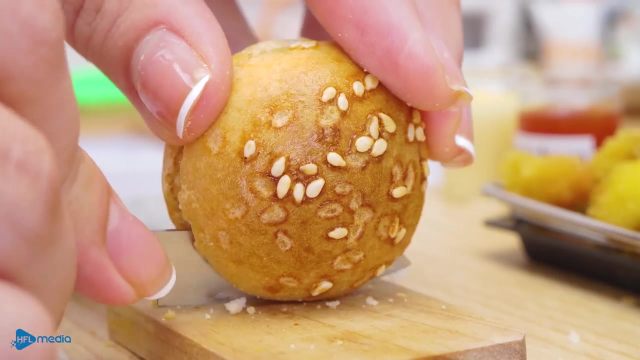 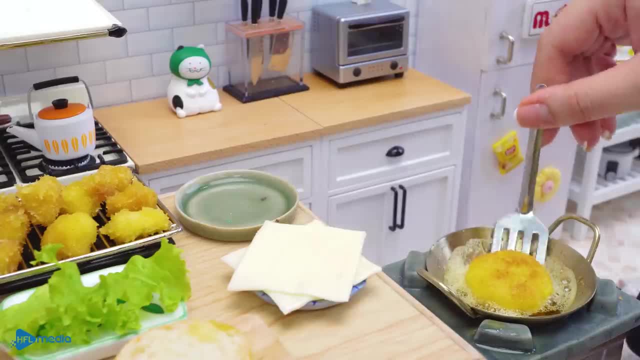 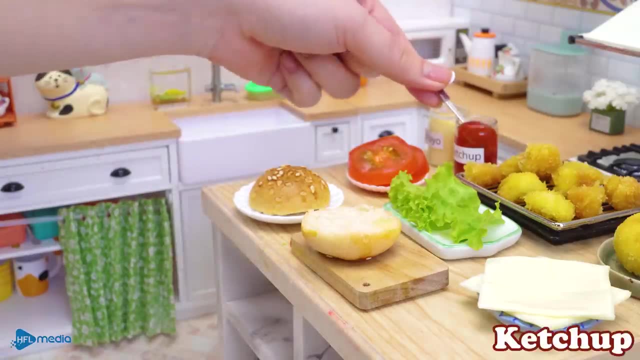 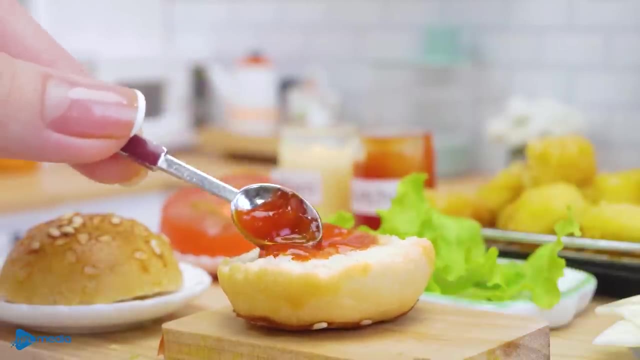 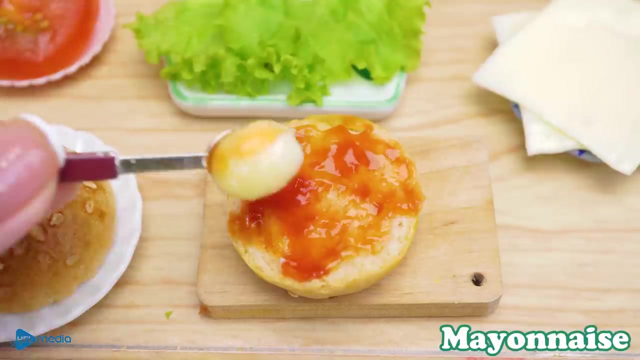 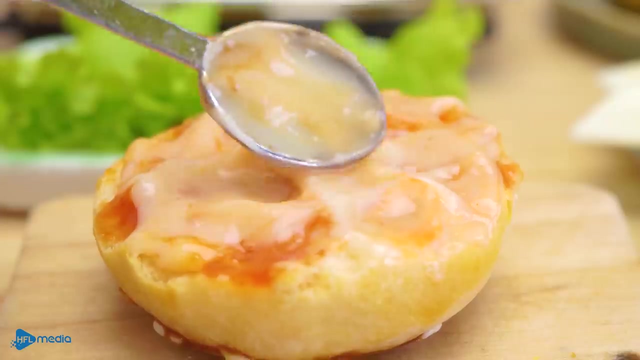 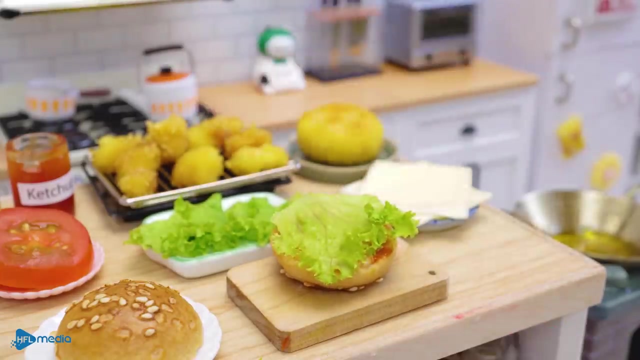 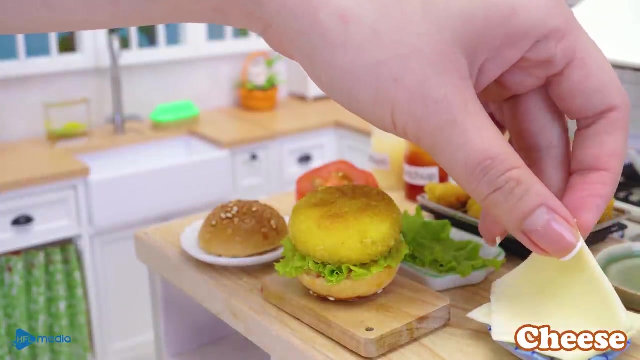 After a while I put a little water. I don't know how to cook, But I think it took me a little longer. So I will indoors, I put it on fire And I will make the sauce. I will add black a little, Add a little salt. Thank you for watching. 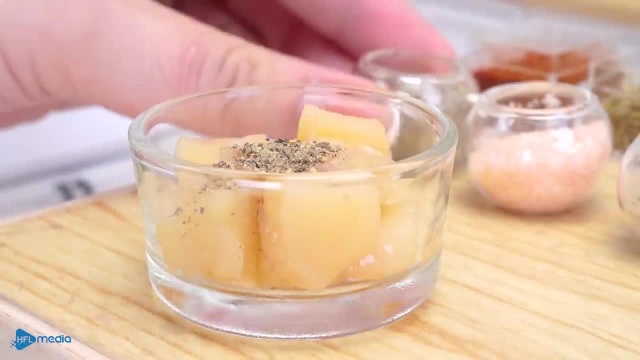 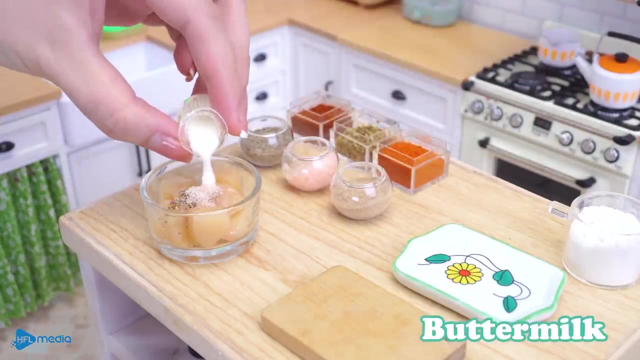 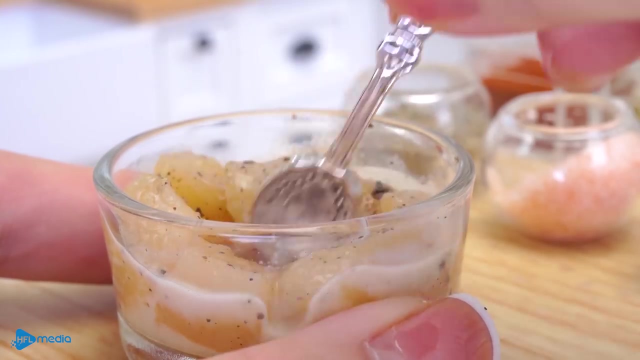 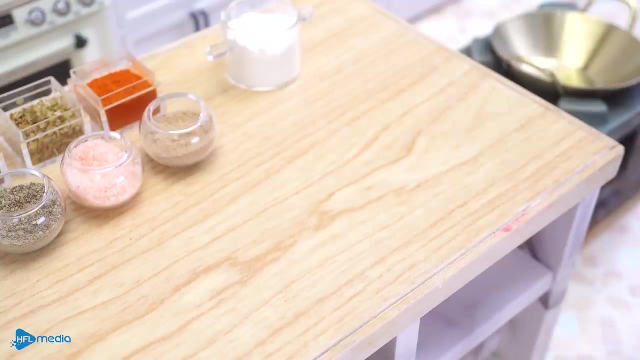 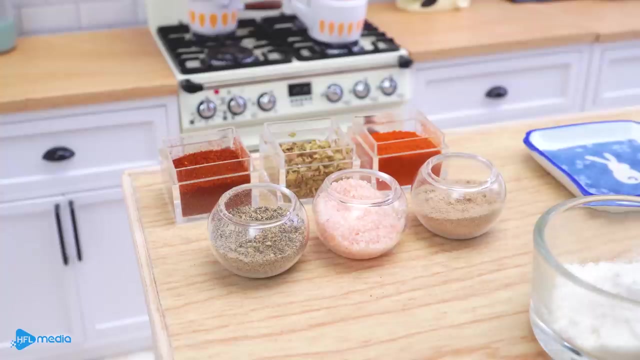 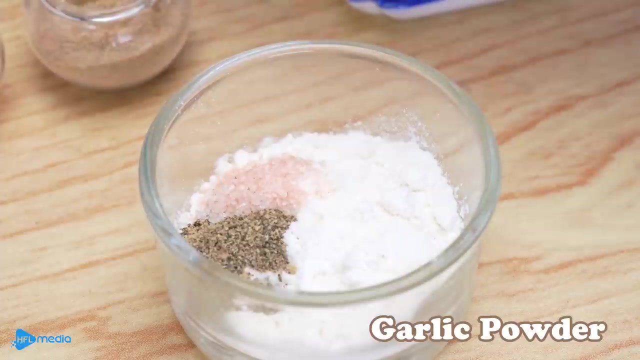 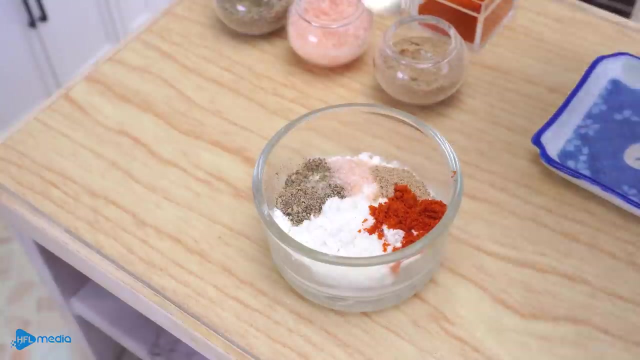 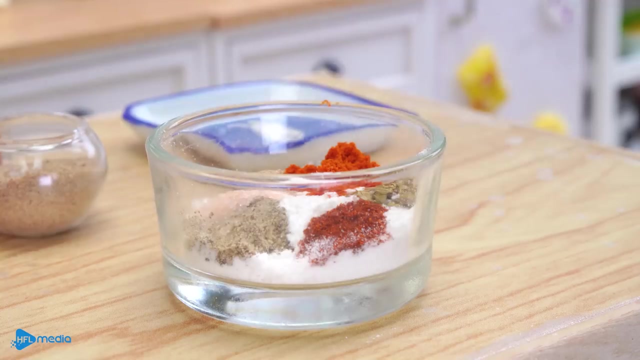 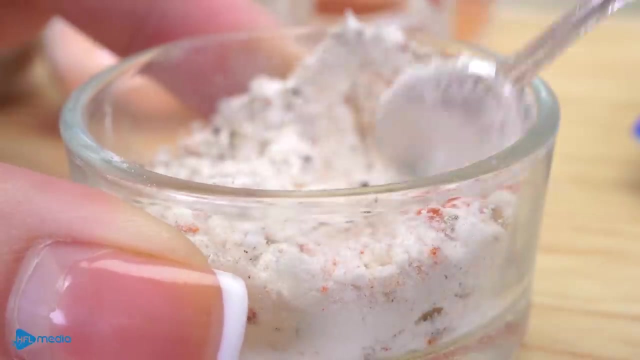 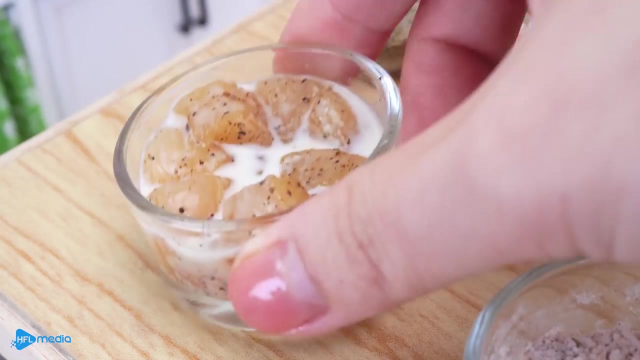 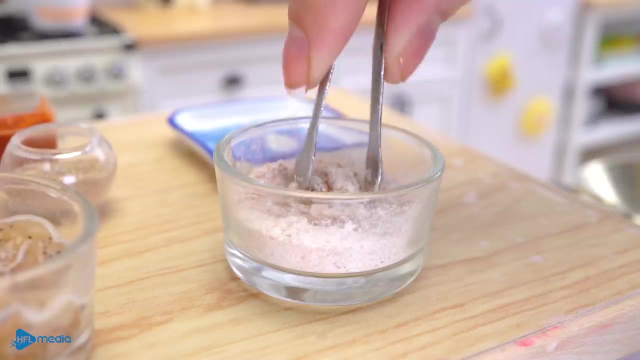 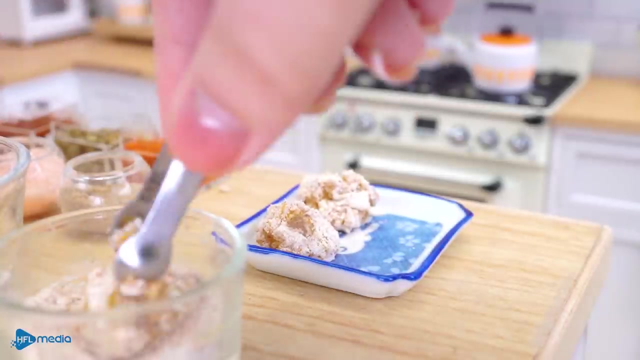 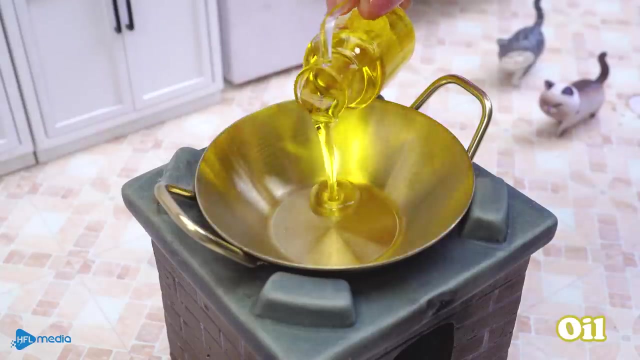 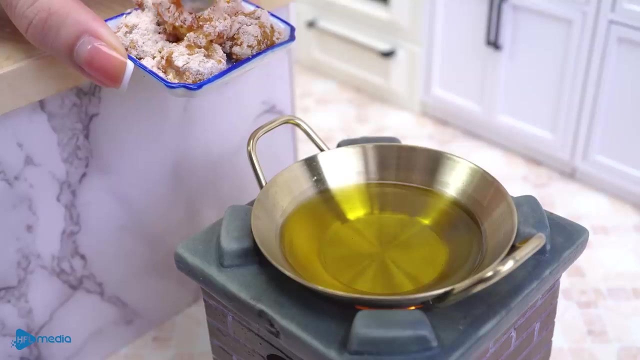 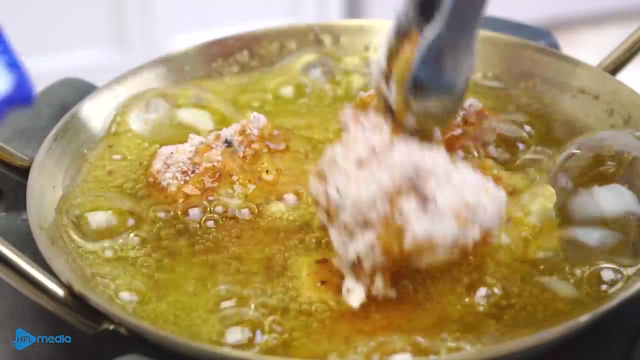 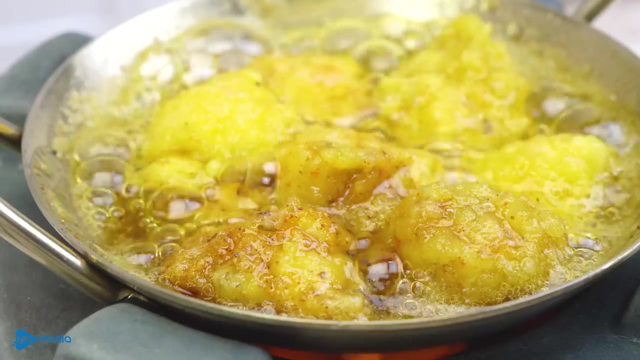 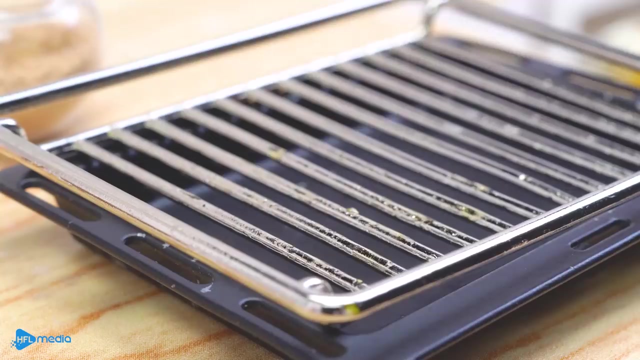 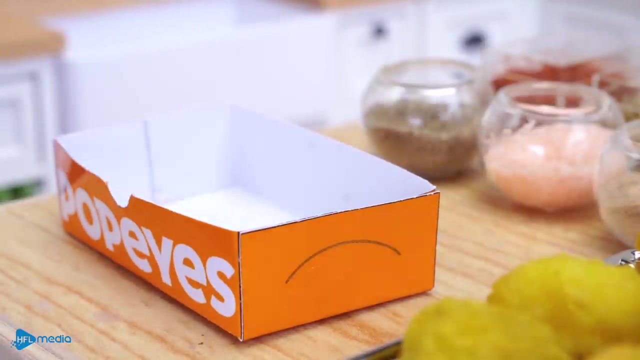 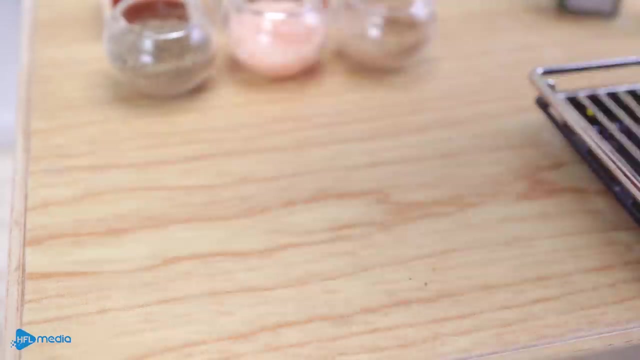 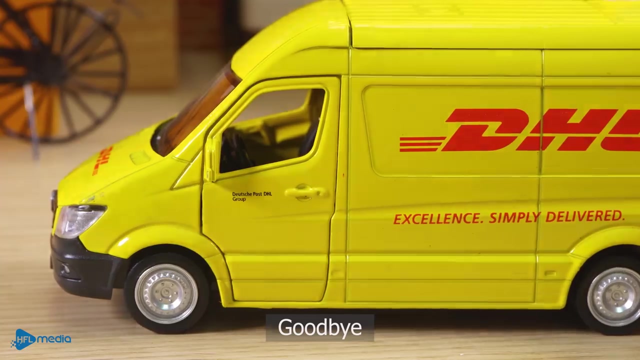 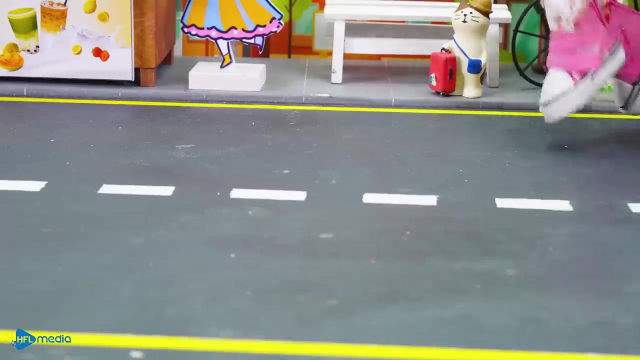 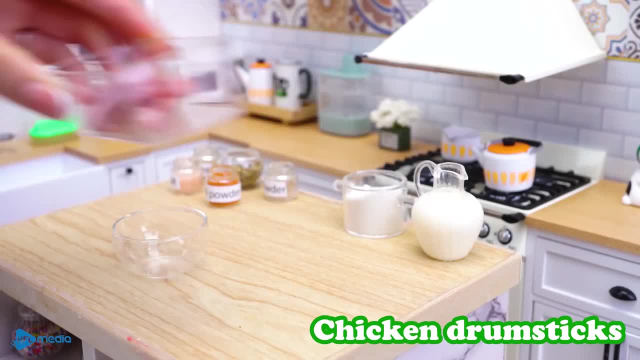 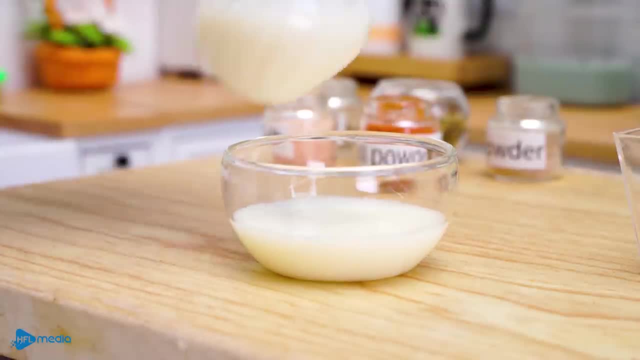 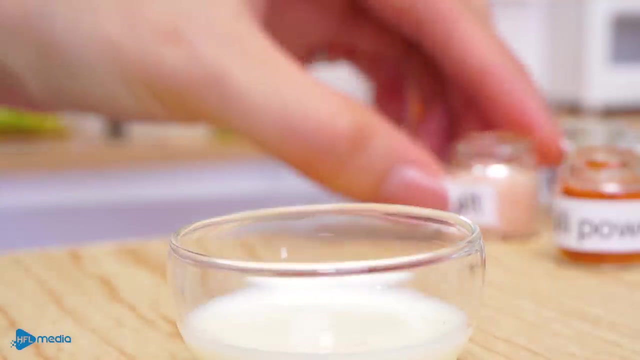 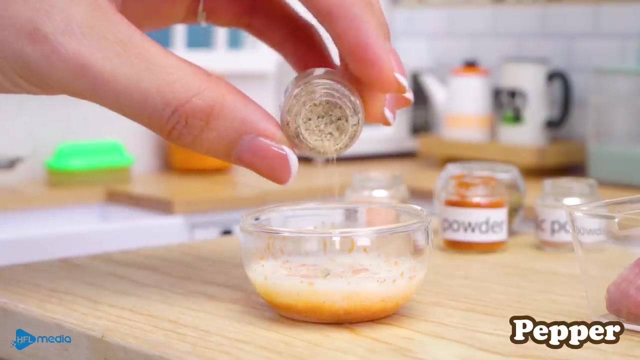 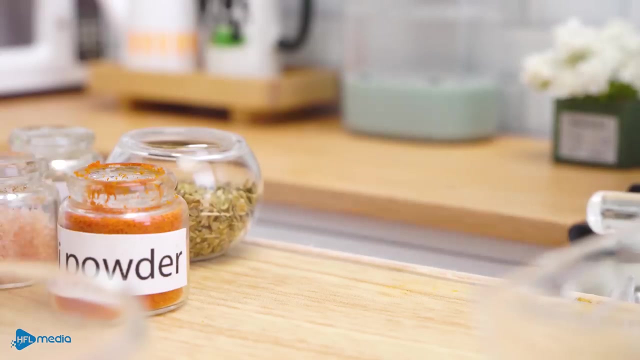 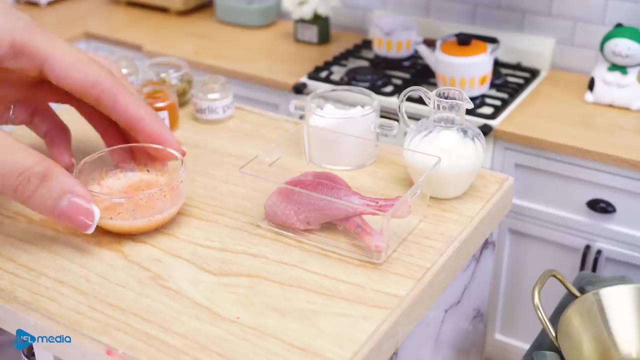 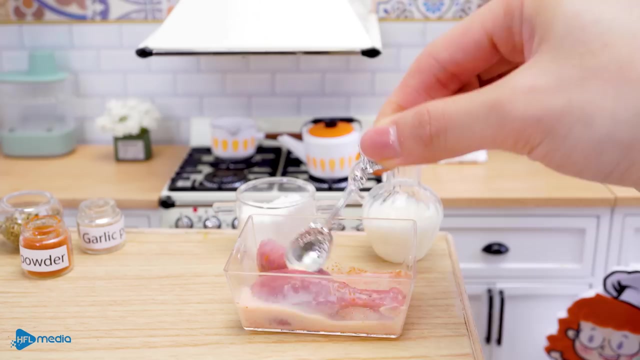 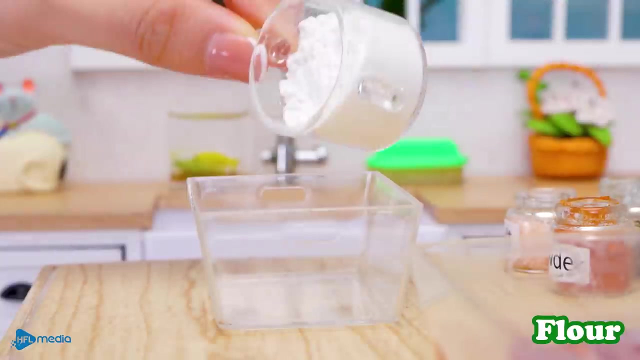 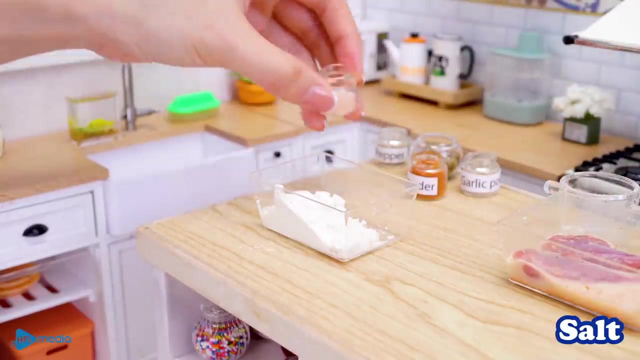 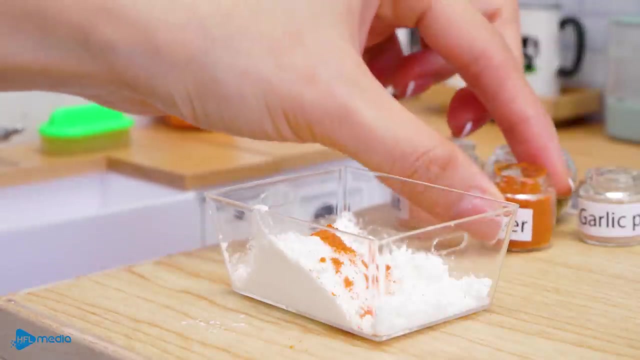 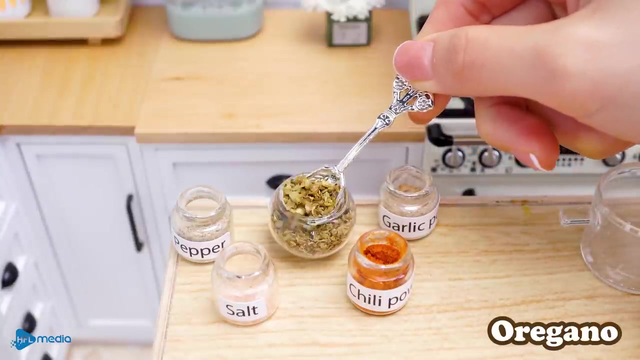 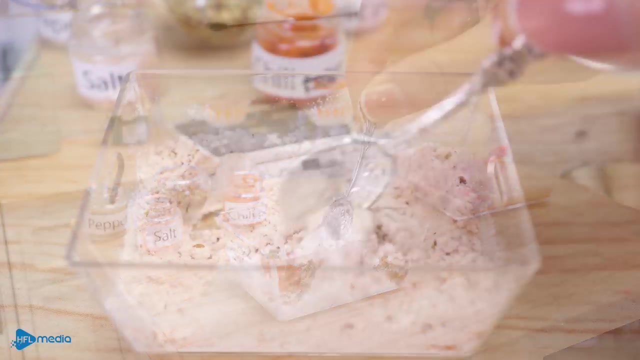 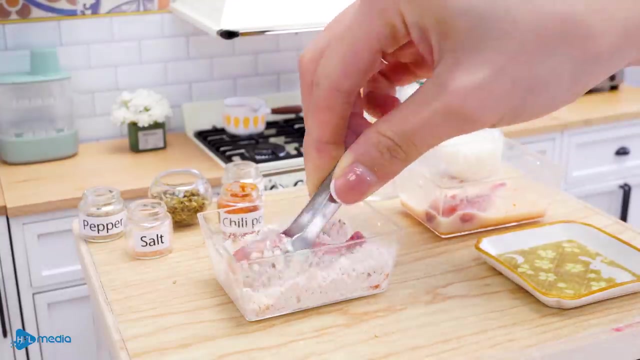 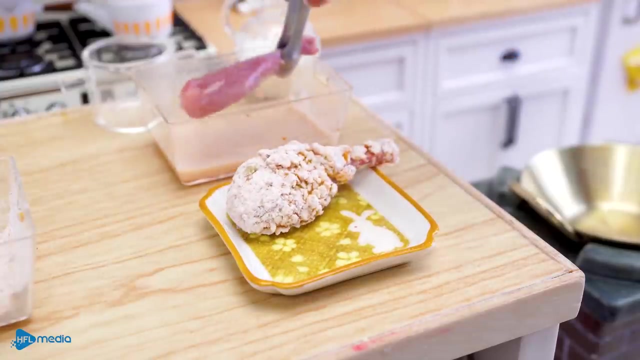 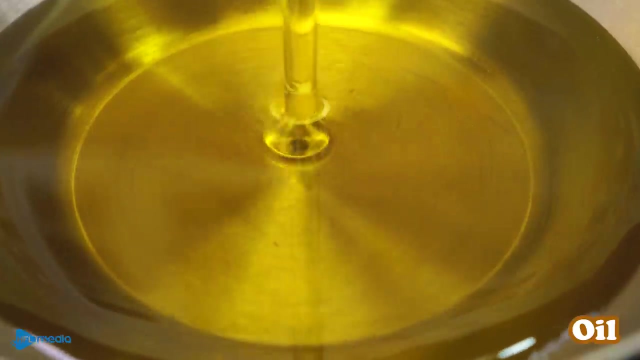 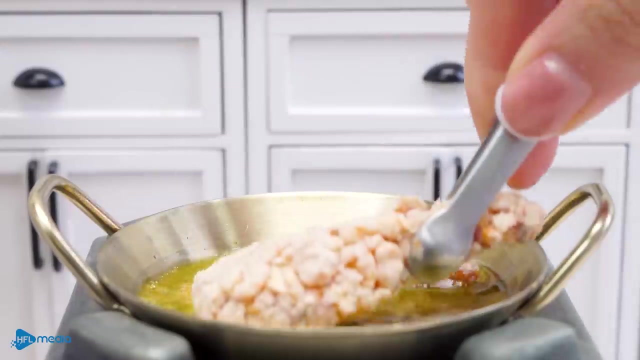 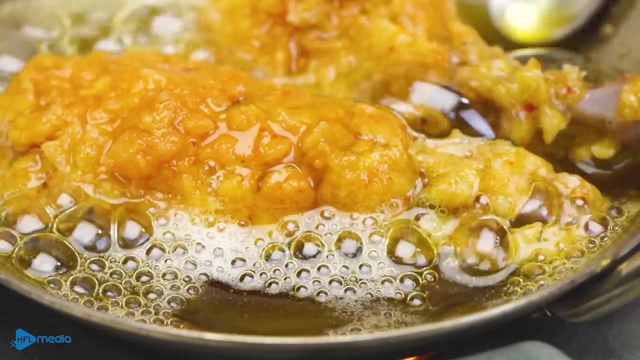 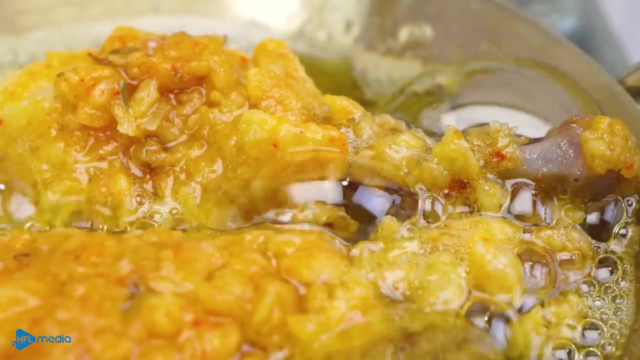 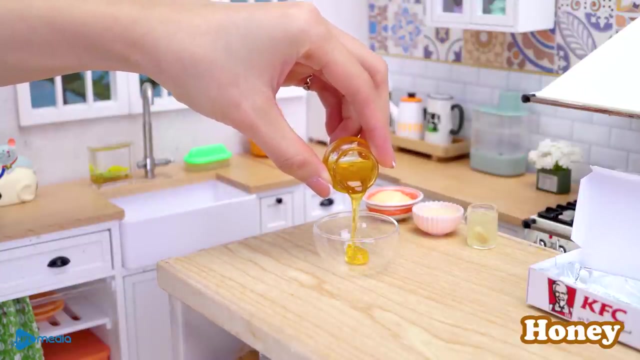 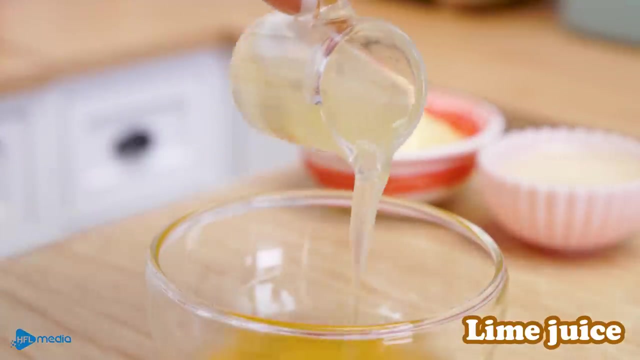 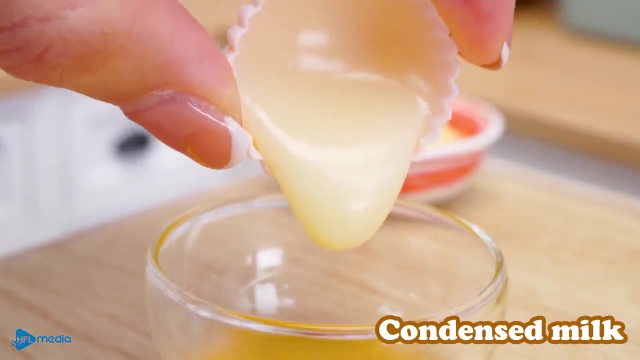 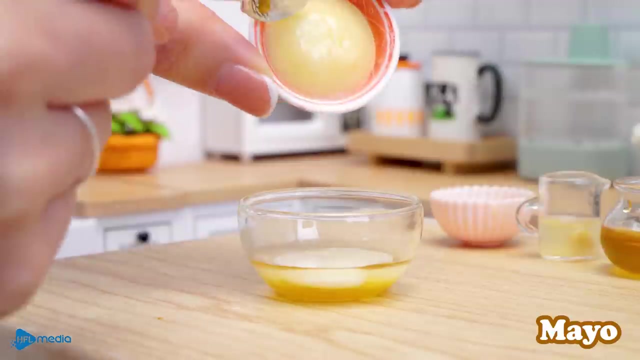 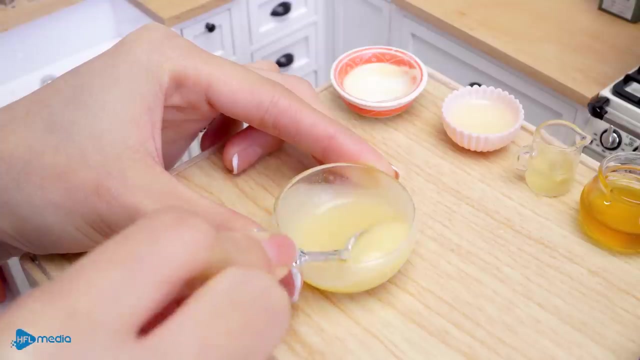 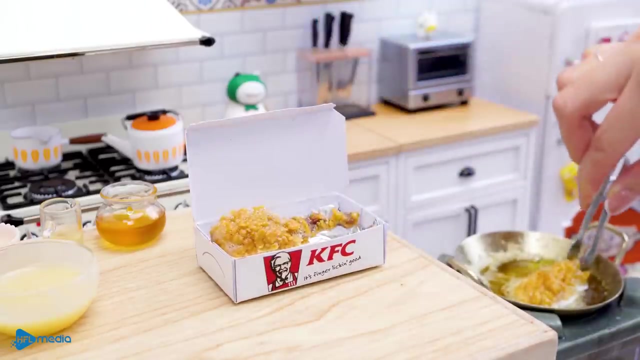 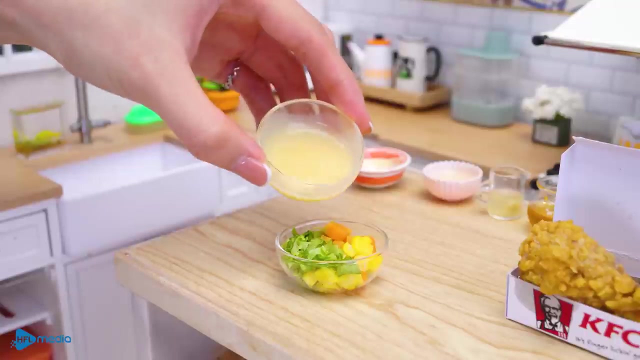 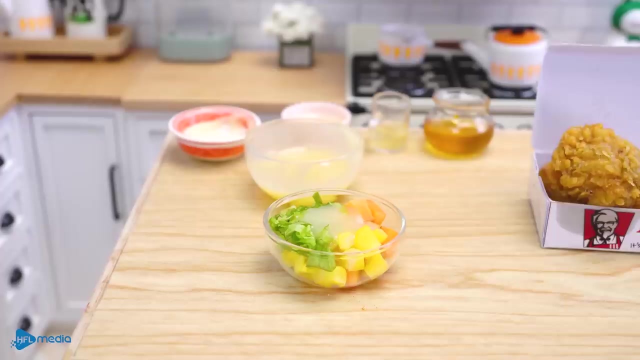 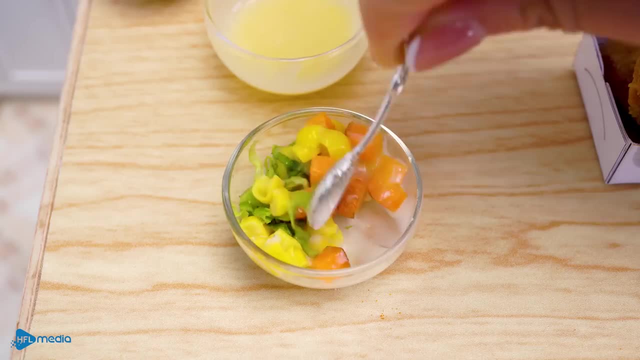 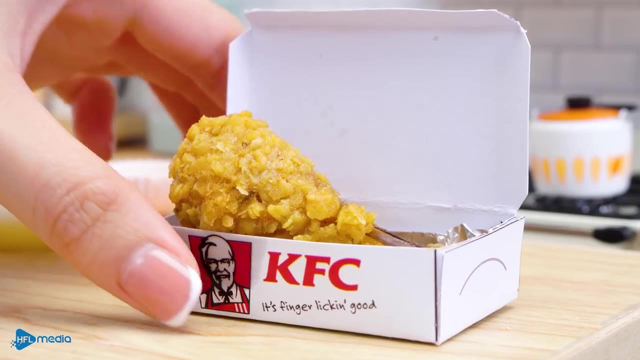 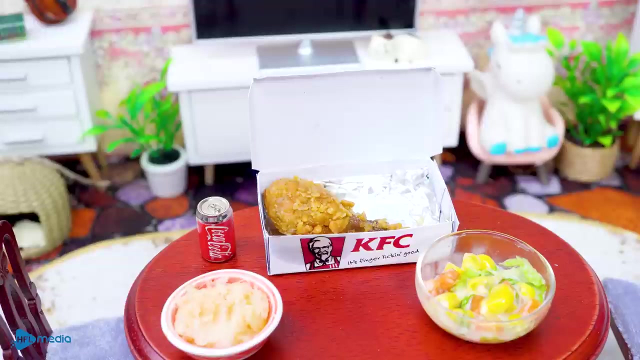 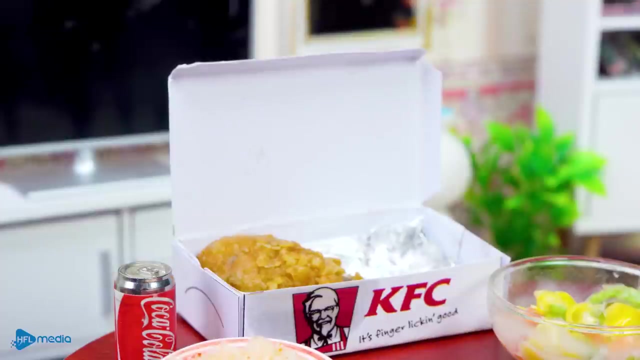 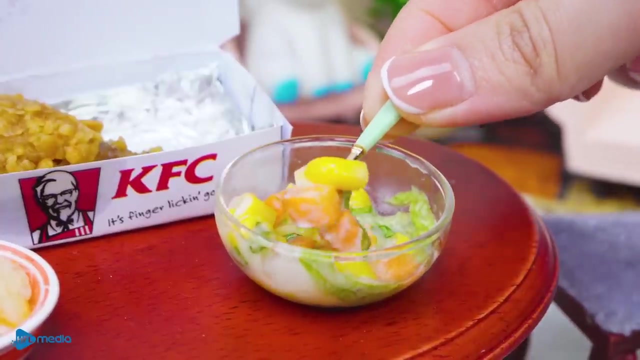 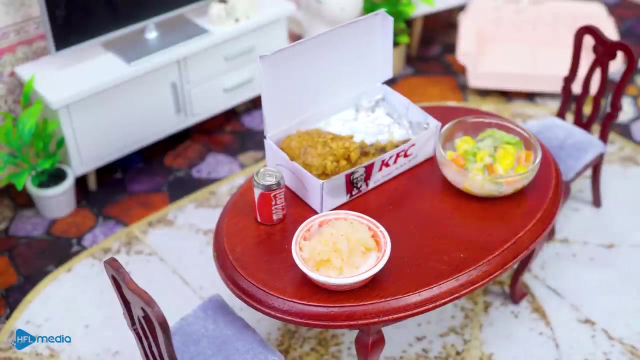 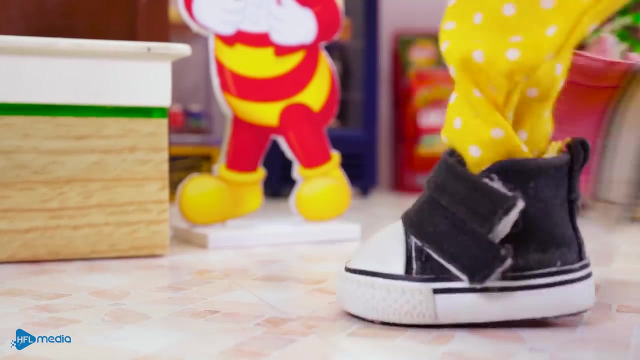 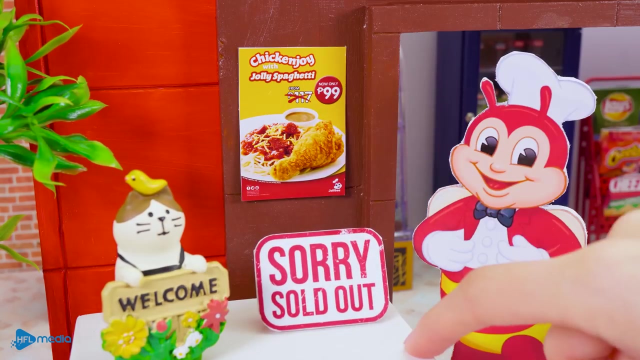 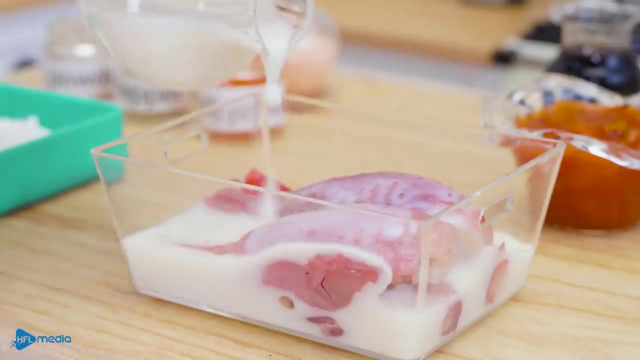 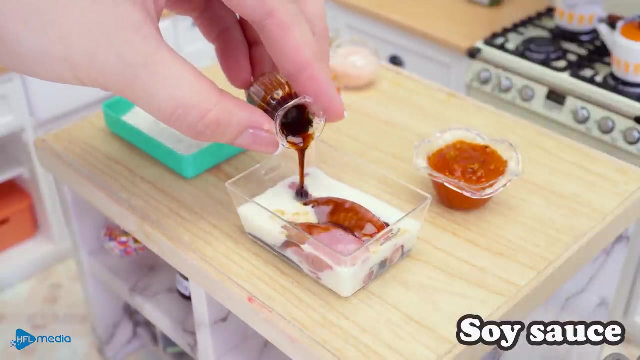 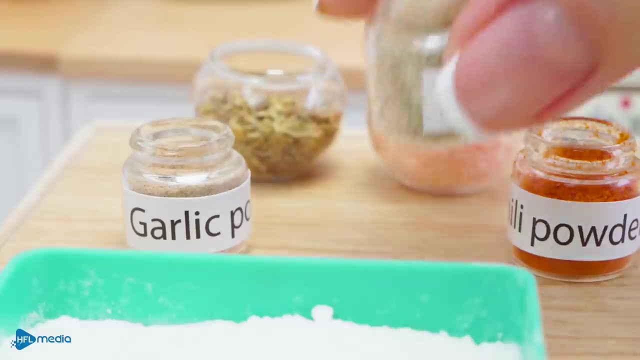 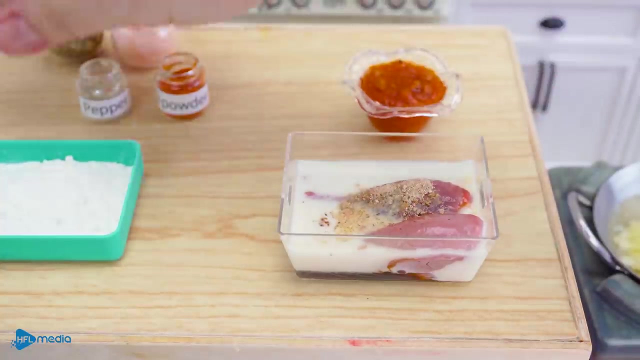 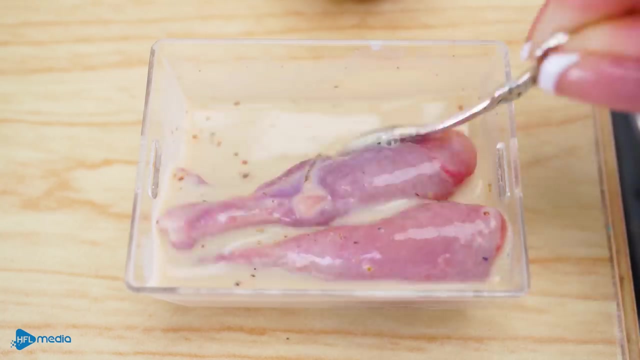 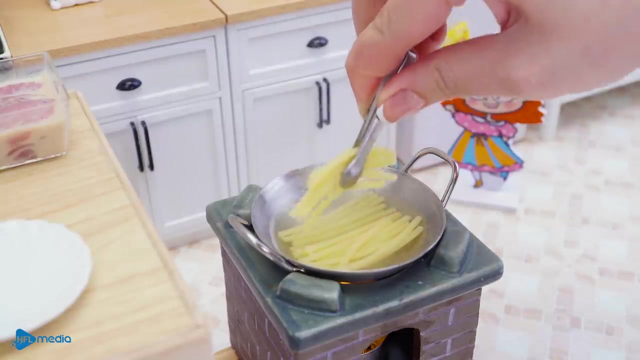 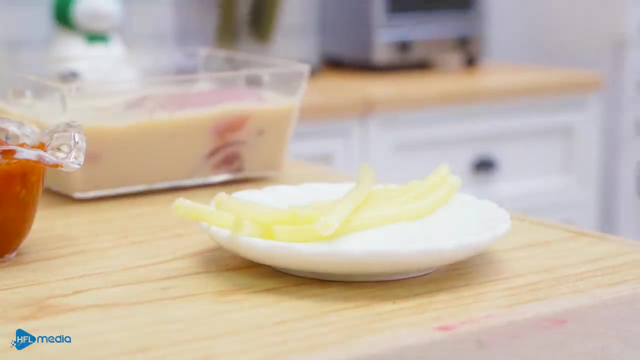 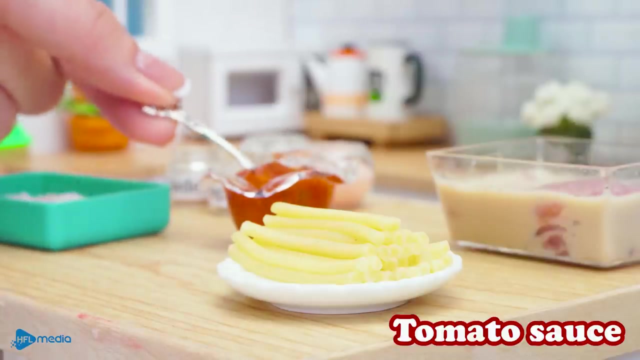 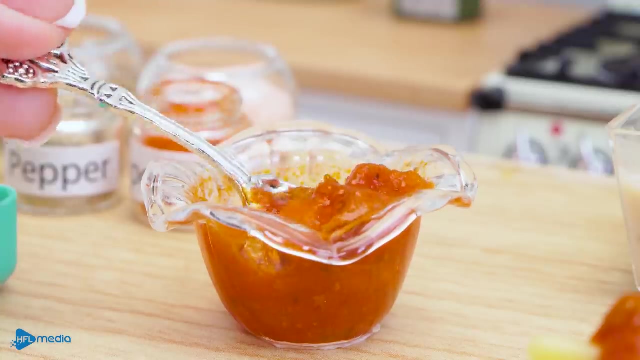 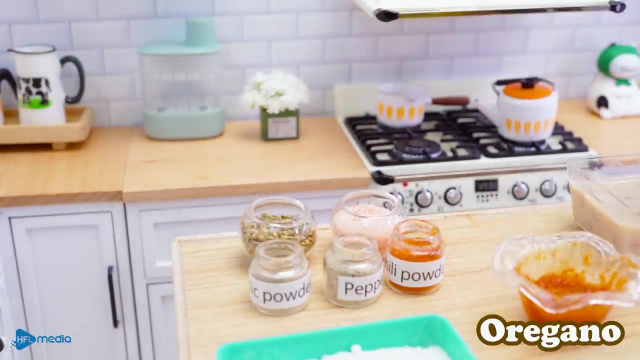 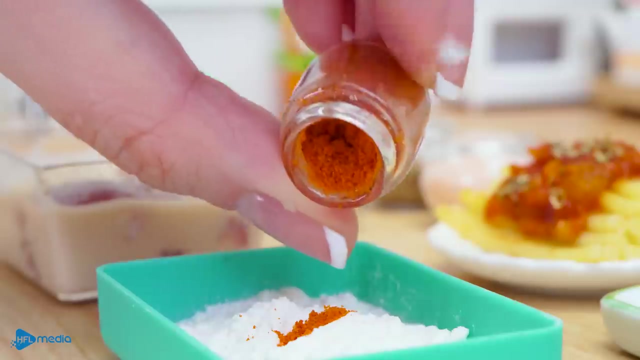 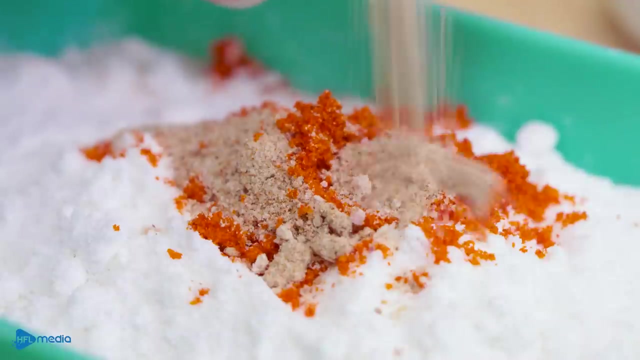 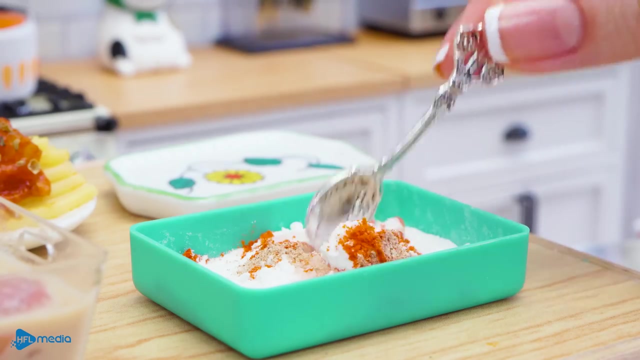 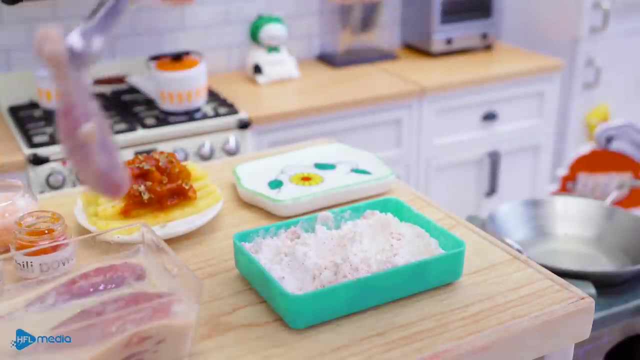 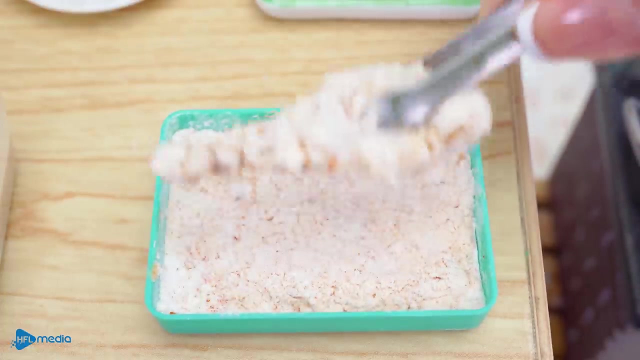 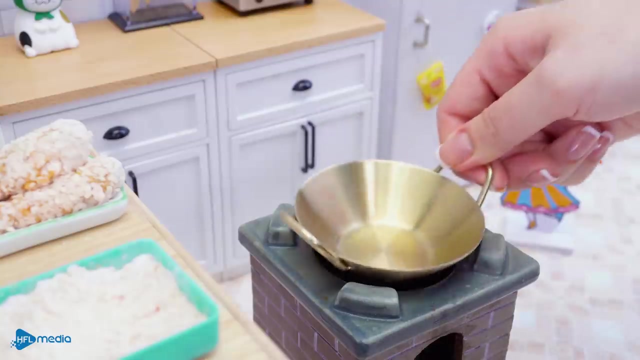 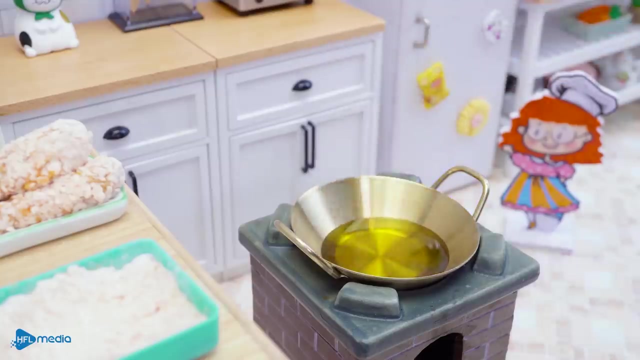 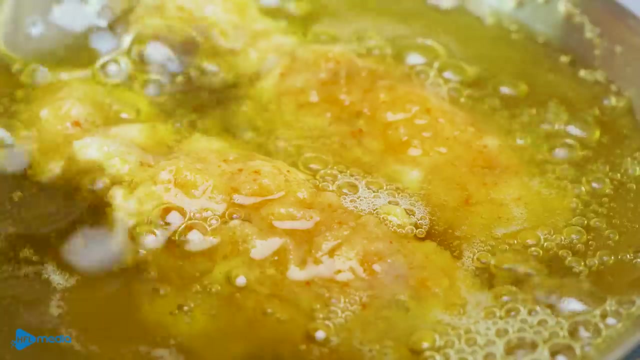 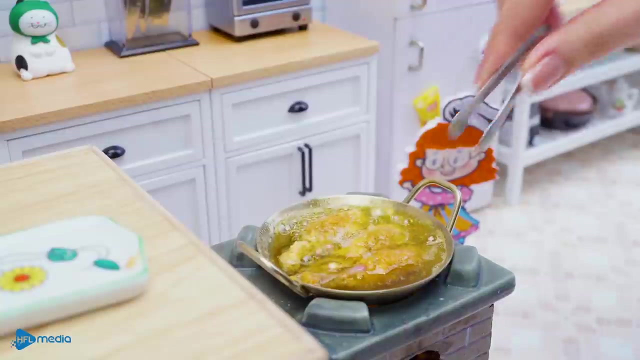 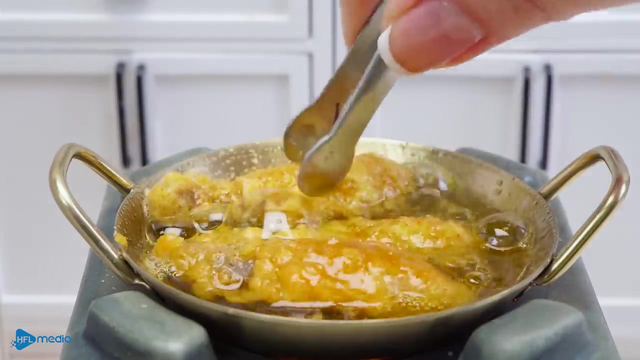 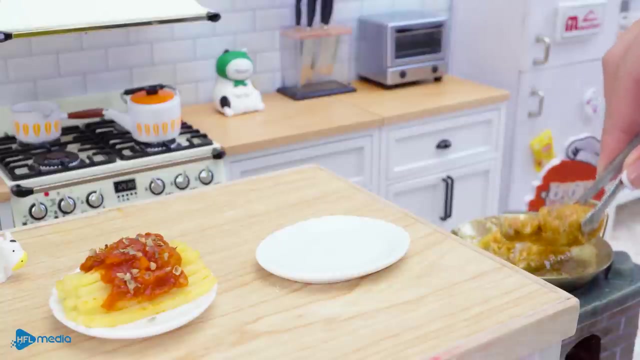 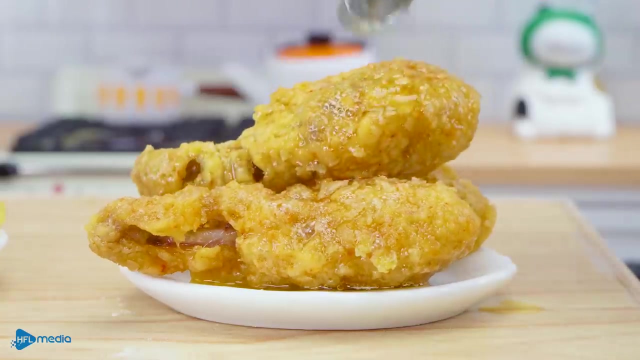 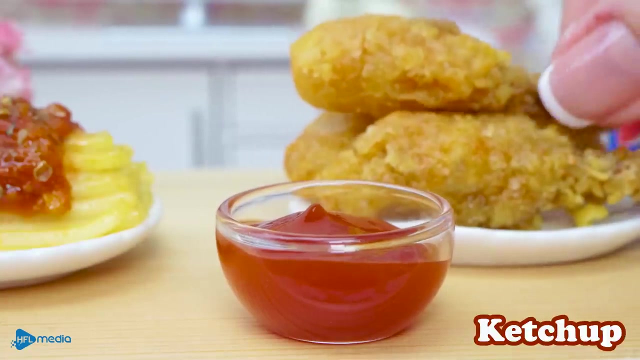 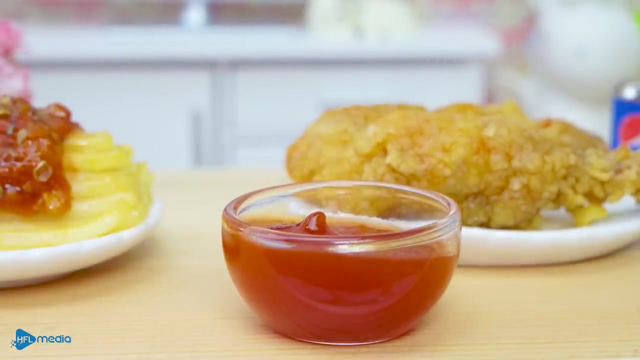 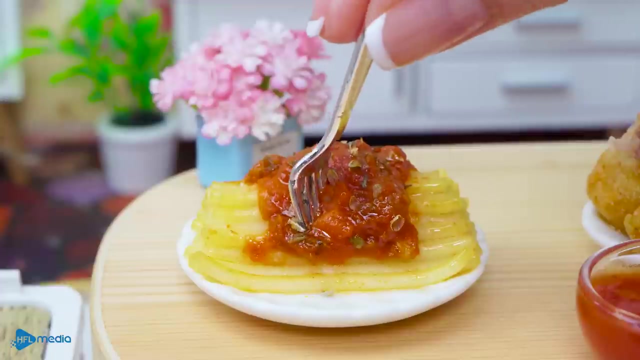 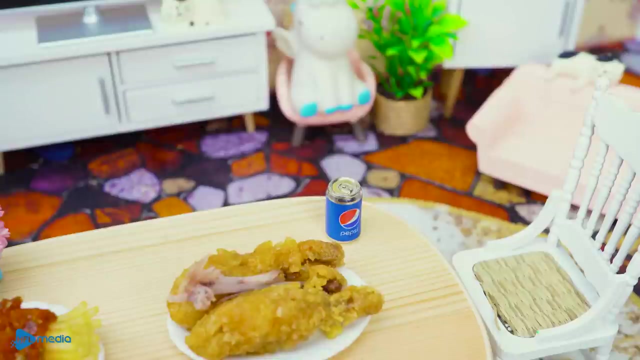 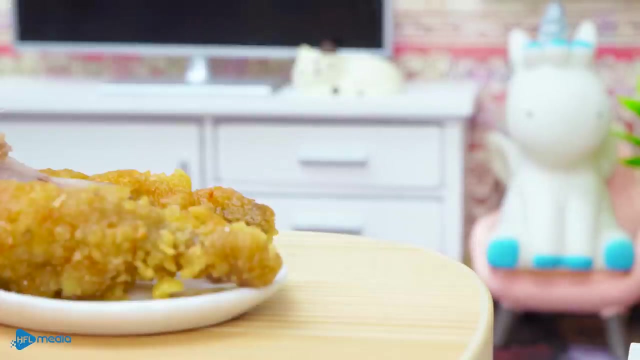 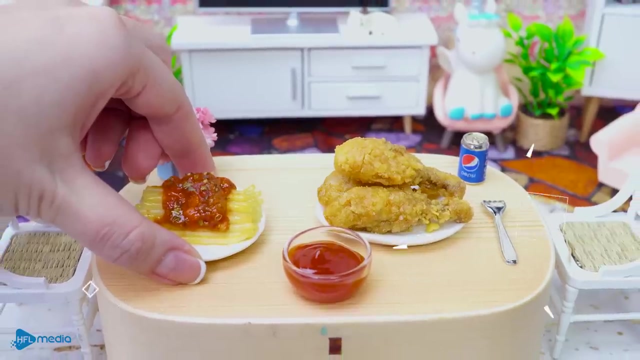